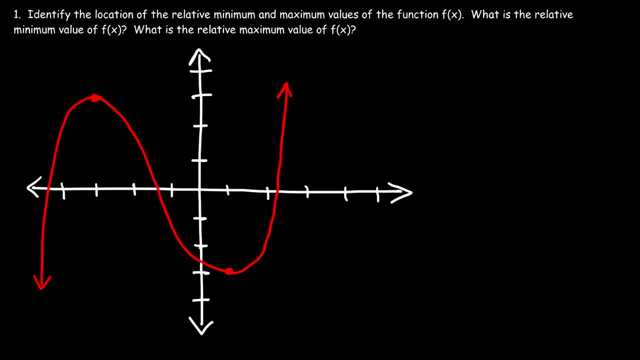 In this video we're going to talk about how to identify the relative maximum and minimum values of the function f of X. So here we have a maximum, a relative max. It's the highest point in that region and over. here we have a relative minimum. 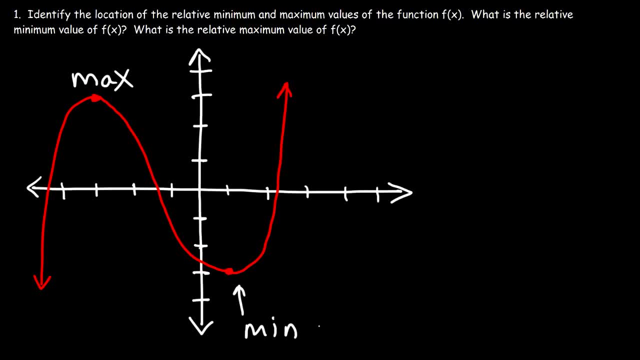 Now the location of these values is associated with the X values. So we have a relative max at X equals negative 3 and we have a relative min at X equals 1.. Now the actual relative maximum value is the Y value that corresponds to this. 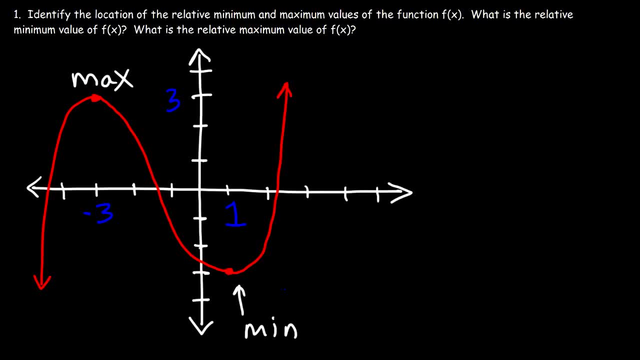 point. So the Y value is positive 3 and here the Y value is negative 3.. So let's say, if we were asked to find the location of the relative maximum, we could say that it's located at x equals negative 3, and the location of the relative minimum we could say it's. 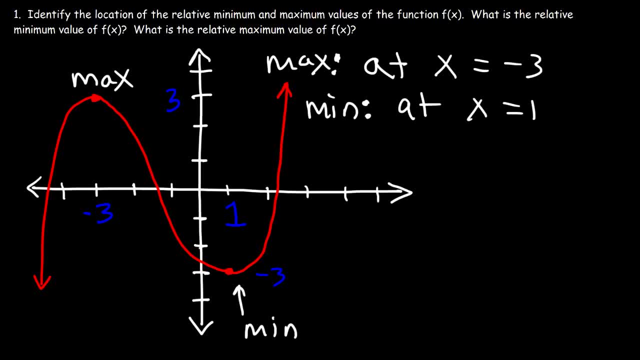 located at x equals 1. and then, for this part, what is the relative minimum value of f, of X? so the relative minimum value that's equal to the y value that corresponds to that point, so that's negative 3, and the relative maximum value is the y value that corresponds to that point, which is positive 3. let's try. 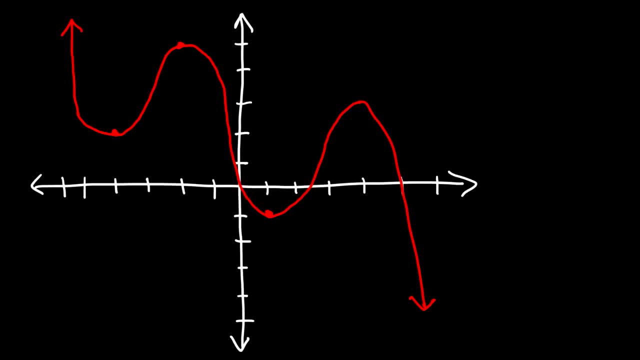 another example. so identify all of the relative extreme values and minimums, the maximums, the location and their actual values. so here we have a minimum and we have a relative maximum, a minimum and another maximum. so the first relative minimum is located at an x value of negative 4 and the second one is located at an x value of 1, the